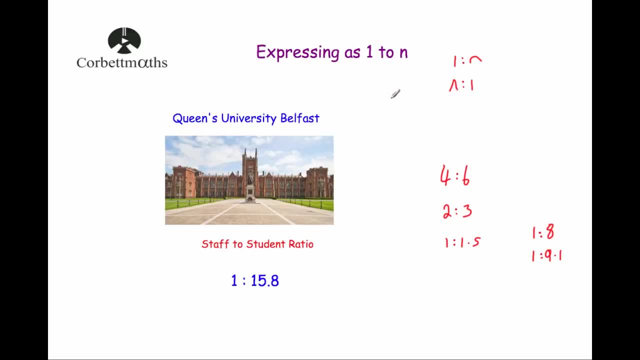 Okay, so expressing ratios in the format 1 to n, it's really useful for comparing them, Sort of to explain why whenever I was at school, we were asked to research the universities we were interested in going to. Whenever we'd done that, we were given lots of books and one of the statistics that I kept on seeing was the staff-to-student ratio. 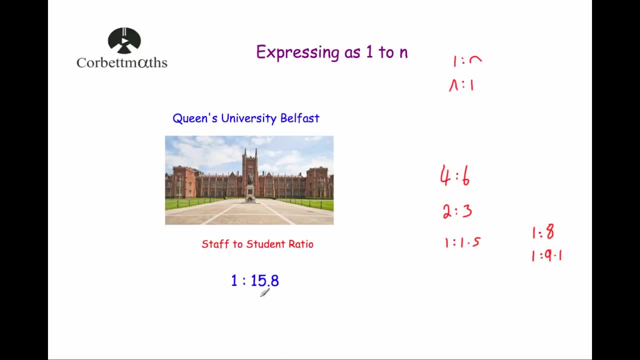 In other words, for one member of staff, how many students there were at that university. Now, the university I went to is Queen's University in Belfast, and I've just Googled this this morning And I thought: well, I'm going to go to Queen's University in Belfast. 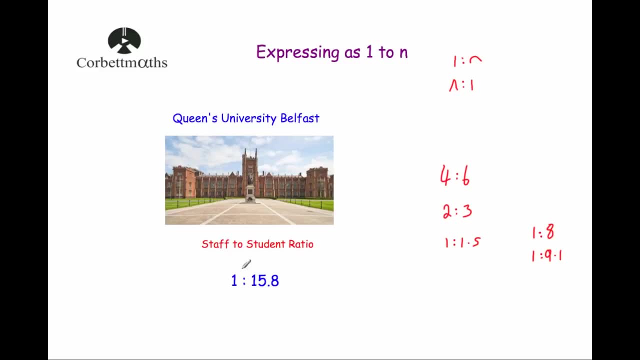 And I thought: well, I'm going to go to Queen's University in Belfast And I found that the staff-to-student ratio currently there, from what I've seen, is 1 to 15.8.. Now, whenever I was deciding to go to university, I wanted this to be quite a good ratio. 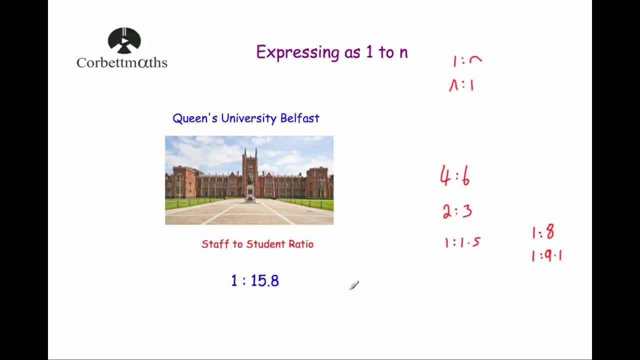 In other words 1 to and a low number. okay, I didn't want a sort of a ratio 1 to 40, because I would have felt that was too many students to staff to sort of get you know sort of personalized help from the staff there at the university. 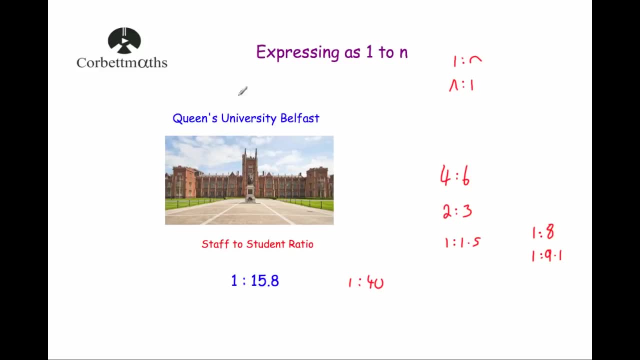 So this ratio, staff-to-student ratio- whenever I chose Queen's, I chose sort of Queen's on the merit of the university being a great university, But also the fact that I was going to go to a university. that was quite a good ratio. 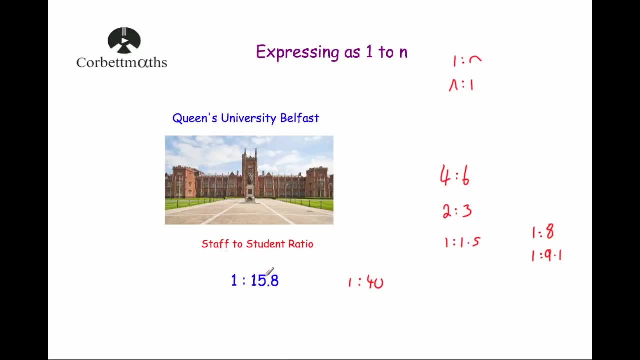 But also the fact that I was going to go to a university. that was quite a good ratio. But also the fact that I was going to go to a university- that was quite a good ratio, But also the fact that I had a really good staff-to-student ratio meant that I could get the support you know from the staff there at the university while studying. 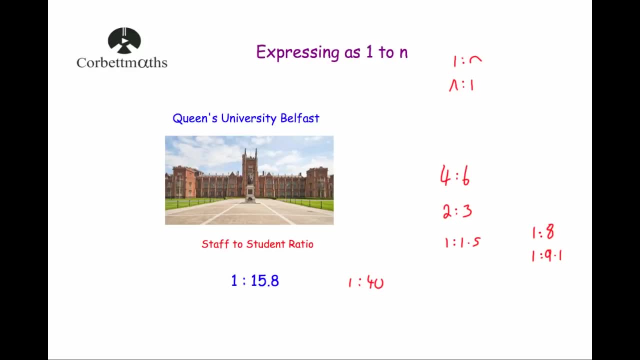 Okay. So this format 1 to N can be very useful for comparing. I'll show you how useful it can be to compare. I've created up a little scenario here where we've got Charlie, who's a striker, who's played 10 football matches and he's scored 13 goals. 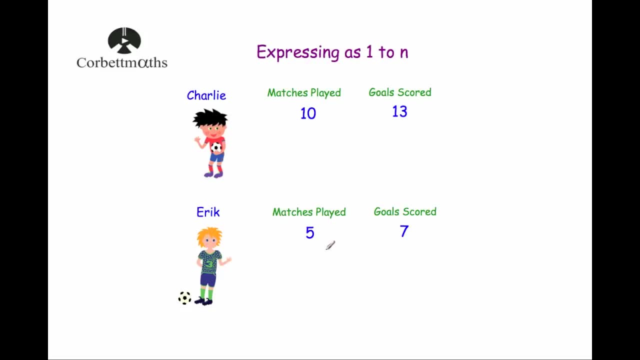 And Eric. he's also a number striker and he's played 5 matches and he's scored 7 goals, And what we're going to do is we're going to write that as a ratio. So matches played, Two goals scored. 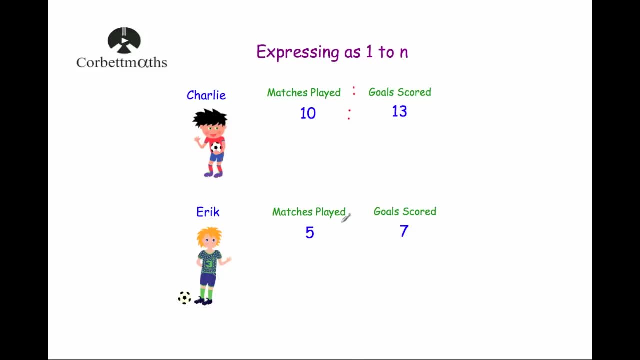 So we've got the ratio here: 10 to 13 for Charlie And for Eric it would be 5 to 7.. Now these two ratios- 10 to 13 and 5 to 7, are both simplified. 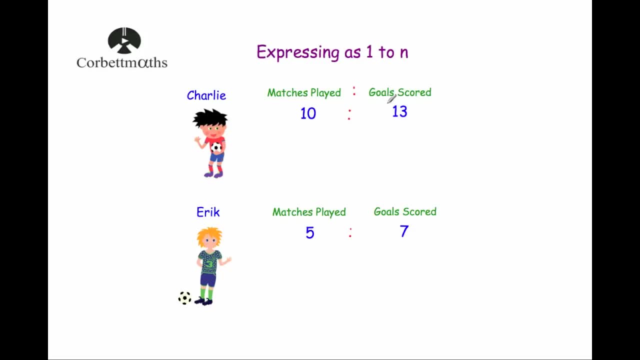 They can't be simplified any further because obviously 10 and 13 have got no other common factors apart from 1. And 5 and 7 have no other common factors apart from 1. So we can't simplify these down any further. 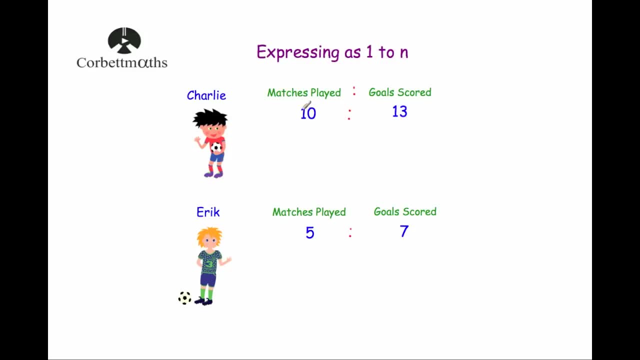 But what we could do is we could write them in the format 1 to N, In other words, make this number at the front 1.. Okay, So we'll get matches. So this is a match that's played for Charlie 1, and for Eric 1.. 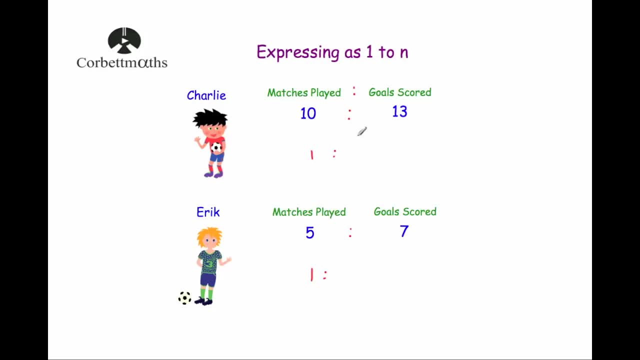 And what we're going to do is we're going to simplify them down to this format: 1 to N. So if it was 10 to 13, both of these numbers are going to be divided by 10 so that we get the 1 at the front. 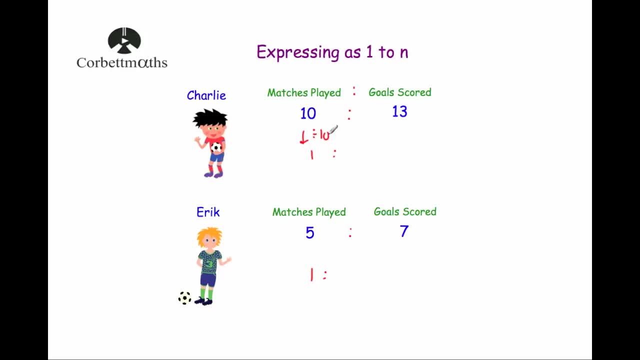 Okay, We want this 10.. Whenever we divide it by 10, we'll get 1.. And we'll also divide this number, 13, by 10.. And 13 divided by 10 is 1.3.. So what that means is that Charlie has a matches played, the goals scored ratio of 1 to 1.3. 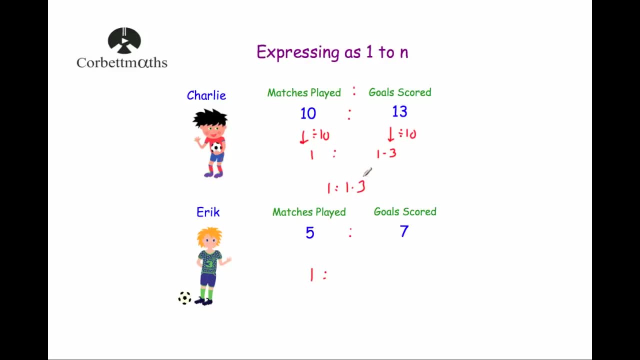 And what that means is for every game he plays, he scores on average 1.3 goals. Now for Eric, he's got the ratio of 5 to 7.. If we divide both of these by 5, so divide by 5 and divide by 5, what we get is: we get. well, 5 divided by 5 is 1.. 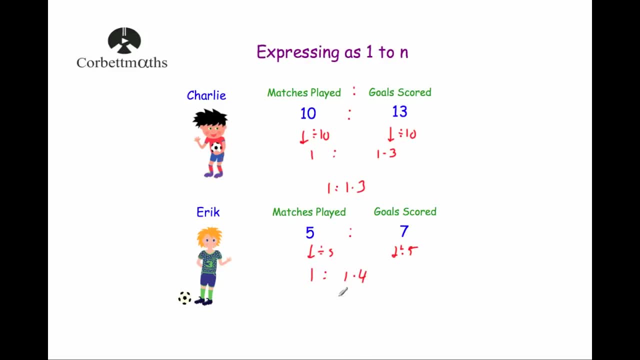 And 7 divided by 5 is 1.4.. So let me say Eric has got a matches played, the goals scored ratio of 1 to 1.4.. So it's a very similar ratio but it's just slightly higher. 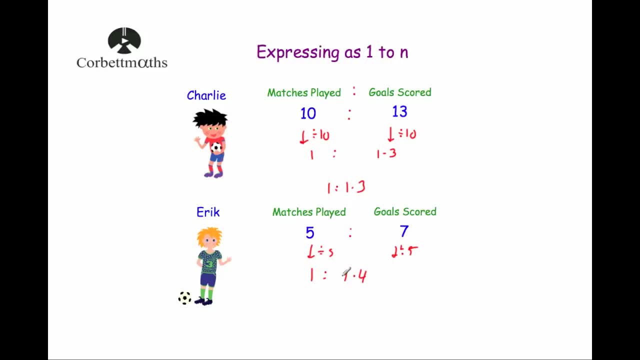 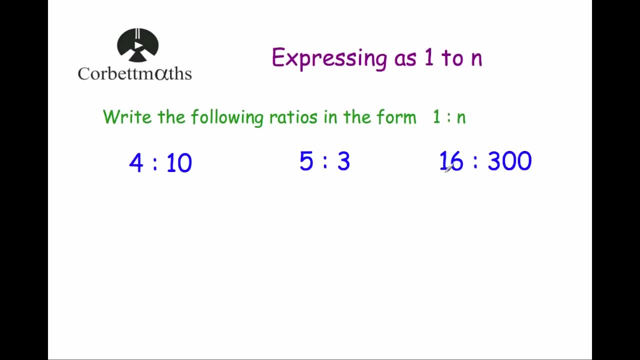 So what it means is that he scores, on average, 1.4 goals per game, compared to Charlie He's 1.3 goals. Okay, let's have a look at some typical questions now. So here we've got some ratios and we've been asked to write them in the format 1 to n. 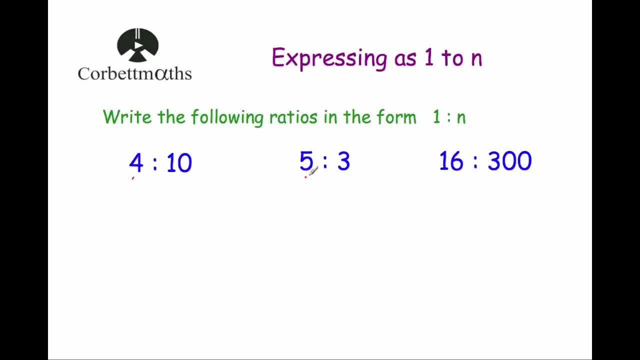 So we want to make the numbers at the front of the ratios- this number, this number and this number- all 1.. And the other values can be whatever they would need to be, So 4 to 10.. So we want a 1 at the front, so we're going to divide both of these by 4.. 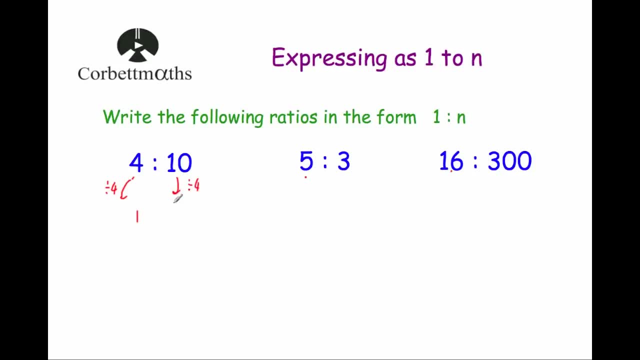 So divide by 4 and divide by 4.. And when we do that, well, 4 divided by 4 is 1. And 10 divided by 4 is 2.5.. So 4 to 10.. 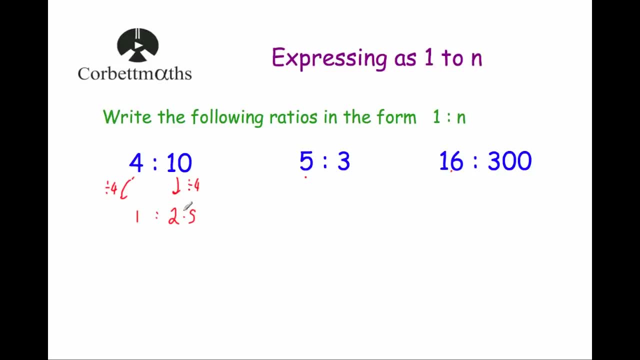 Well, that would be when written in the format 1 to n would be 1 to 2.5.. Okay, next 5 to 3.. So 5 to 3, if we wanted to write that down in the format 1 to n. 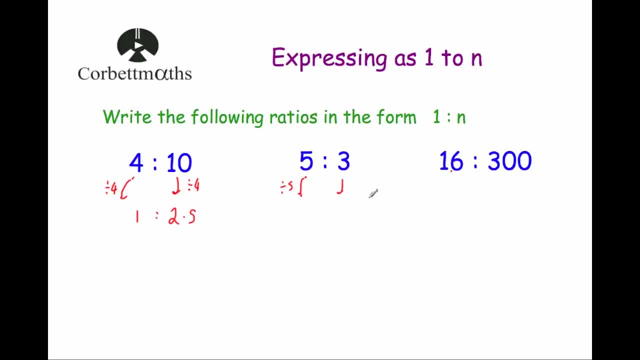 we would divide both of the numbers in the ratio by 5.. So divide by 5 and divide by 5.. And that would give us 1,, 2, and 3 divided by 5 is 0.6.. So 1 to 0.6.. 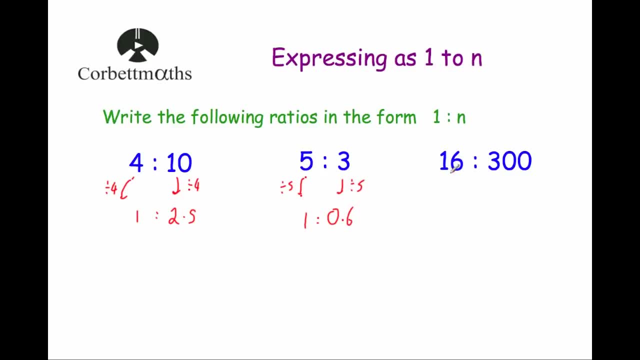 And our last one, 16 to 300.. So we would divide both numbers in this ratio by 16.. So divide by 16. And divide by 16, because we want the number at the front to be 1.. 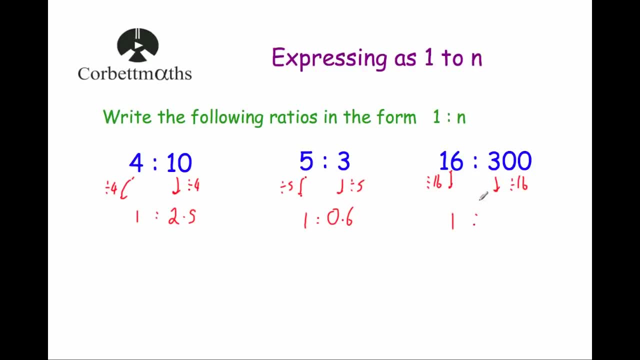 So 16 divided by 16 is 1. And 300 divided by 16.. Off the top of my head I think it's 18.75, but I'll just quickly check on my calculator: 300 divided by 16 is 18.75.. 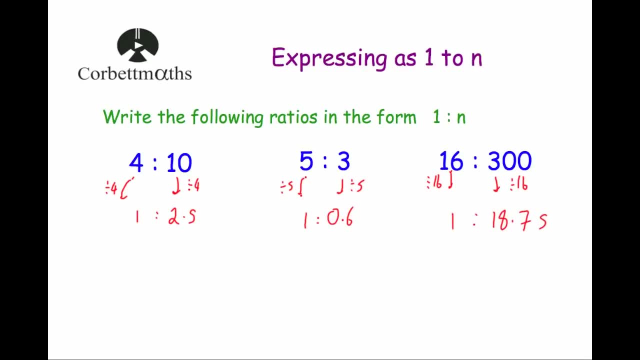 Great. So we have written all these ratios in the format 1 to n. Now what we're going to do is we're going to do some questions where the question is asked, to write the ratios in the format n to 1.. 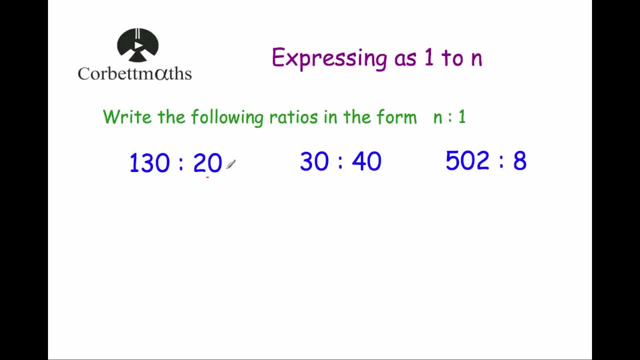 In other words, it wants the second number in the ratio And the ratio to be 1.. So it wants this number to be 1, this number to be 1, and this number to be 1.. So if we've got the ratio 130 to 20,, if we want the second number to become 1, we're going to divide both of them by 20.. 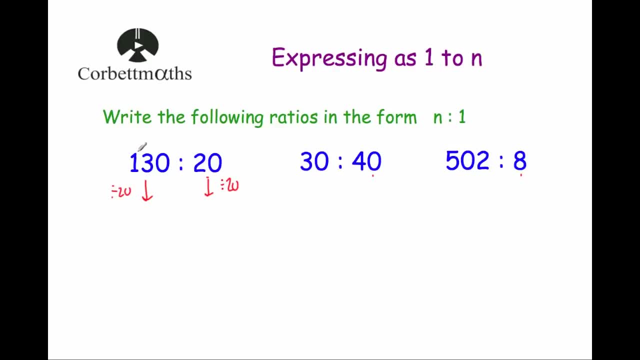 So divide by 20 and divide by 20.. 130 divided by 20 is 6.5.. And 20 divided by 20 is 1.. So 130 to 20 written in the format n to 1 would be 6.5 to 1.. 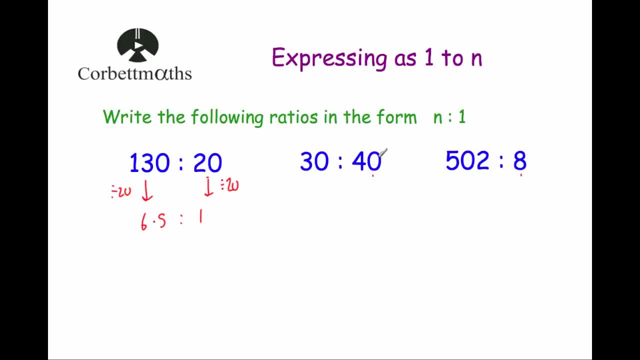 Okay, next, 30 to 40. So we want the second number to be 1.. So we're going to divide both sides by 40. So divide by 40 and divide by 40. And when we do that, 40 divided by 40 is 1 for the second number. 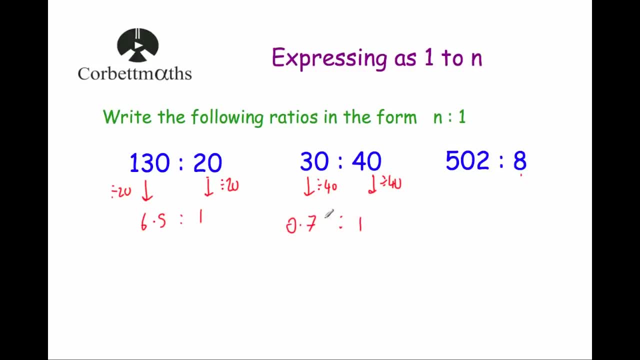 But for the first number, 30 divided by 40 is 0.75.. So 30 to 40 written in the format n to 1 would be 0.75 to 1.. And finally, 502 to 8.. 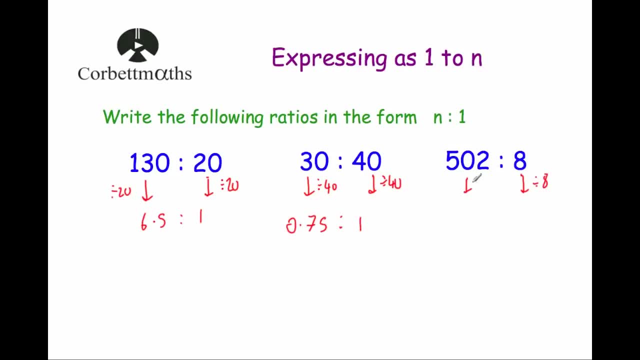 Well, we want the second number- this 8, to become 1.. So we're going to divide by 8 and divide by 8.. When we do that, we get. Well, the second number is going to be 1.. 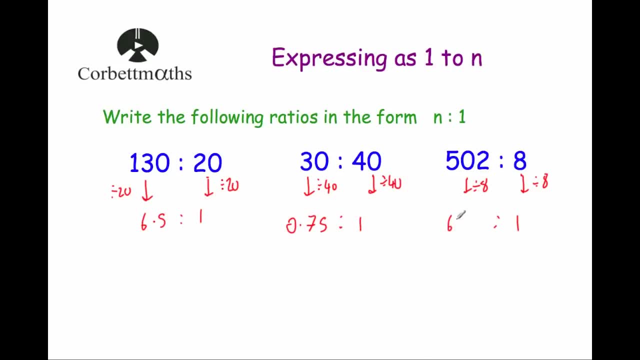 And 502 divided by 8 would be 62.75.. And that's it, Thank you. 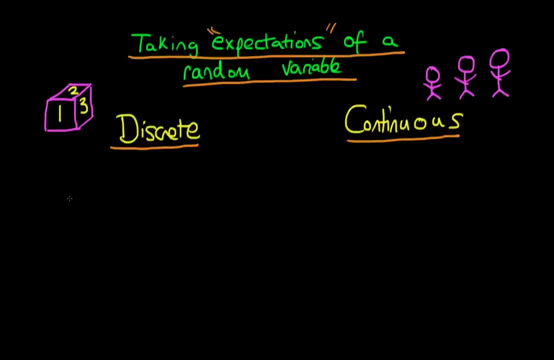 In this video, I'm going to be talking about what we mean by taking the expectation of a random variable, and I'm going to be describing this in both the discrete and the continuous cases. So in a discrete case, the example which I'm going to use here is that of throwing a fair die, So a